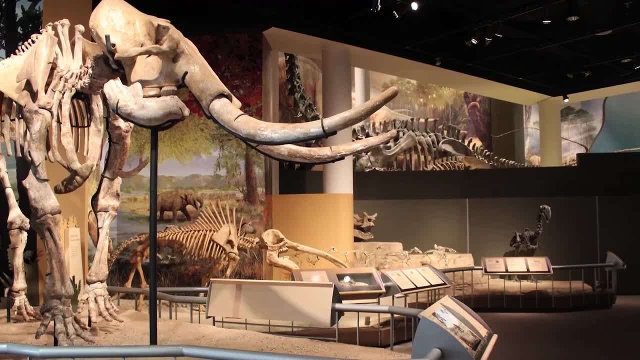 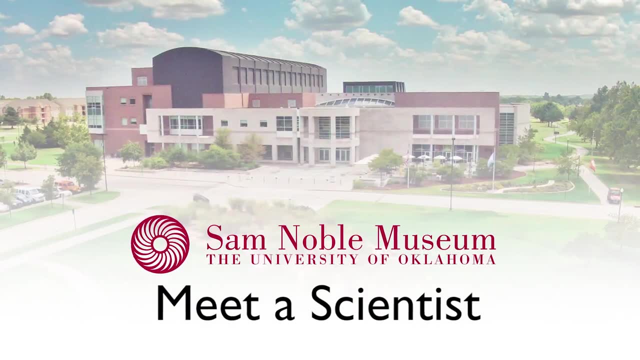 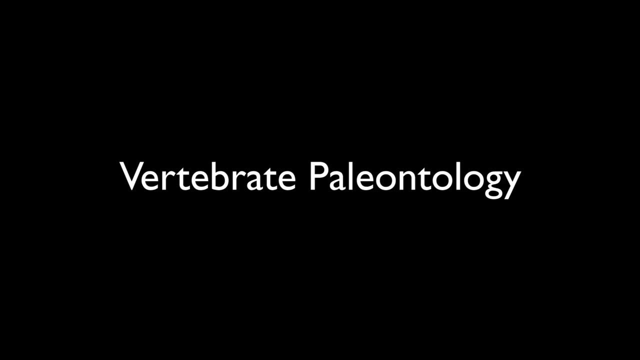 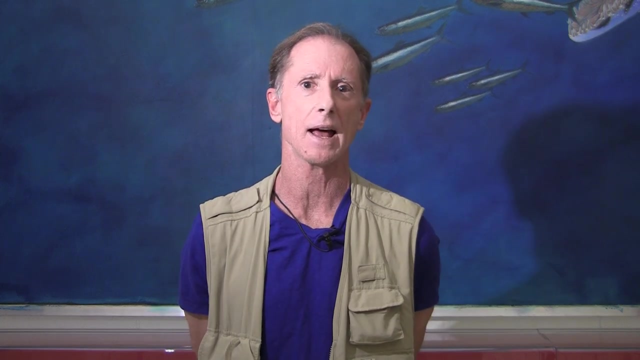 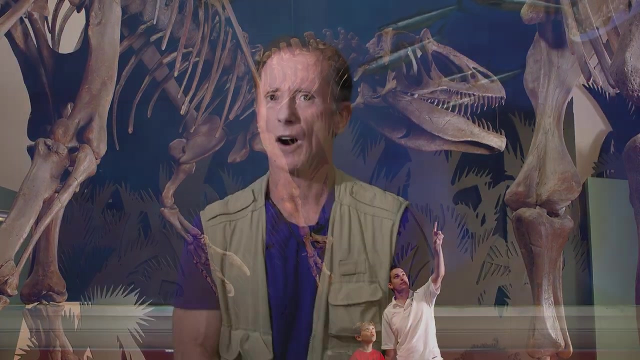 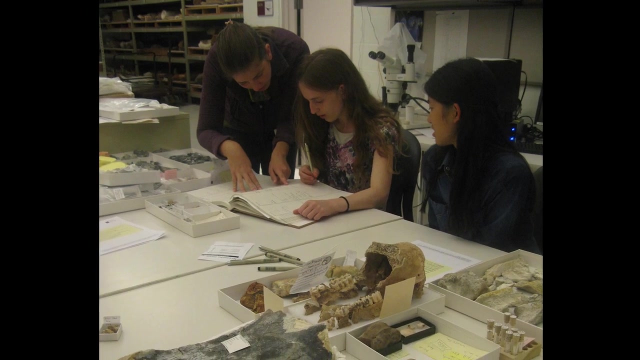 My name is Richard Cifelli. I am a paleontologist. We study life of the past, usually extinct species, based on fossils- fossils that we go out and collect. Our collection is one of the very biggest around, so we teach classes using the real fossils And we are kind of at the intersection of life and earth sciences. 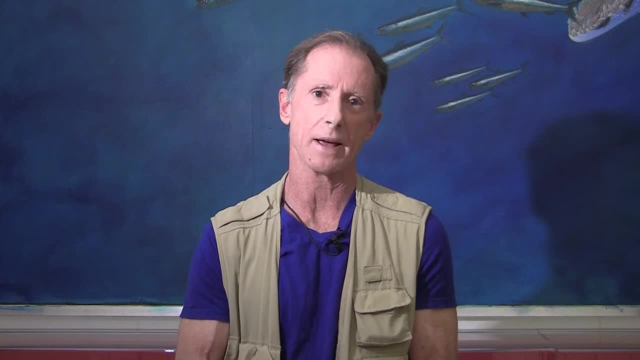 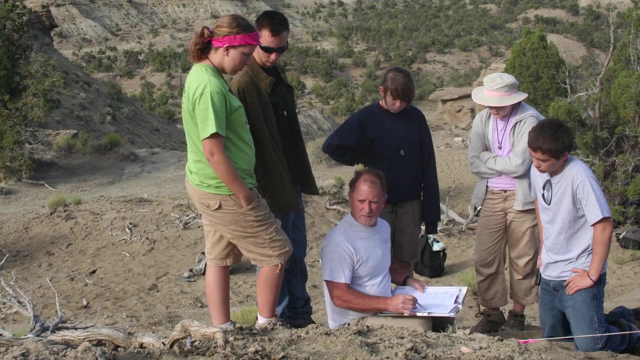 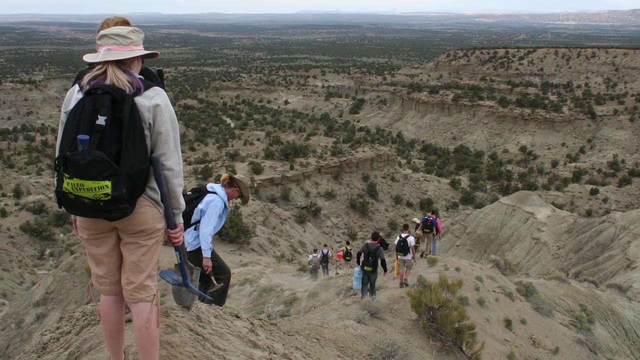 so somebody who studies paleontology would expect to have to take the sort of science track courses: biology, geology, and then the various chemistry and physics. That's all important preparation for a scientist in training. The funnest thing is to be able to go out in the field and find something. 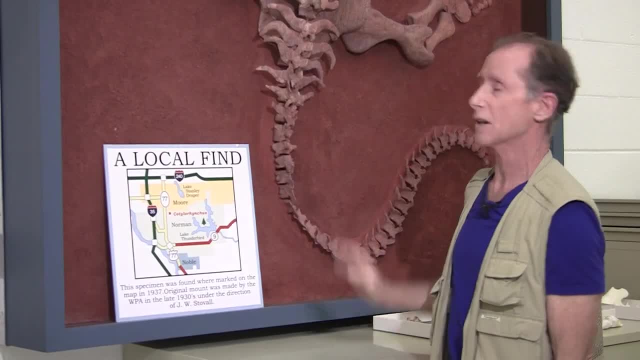 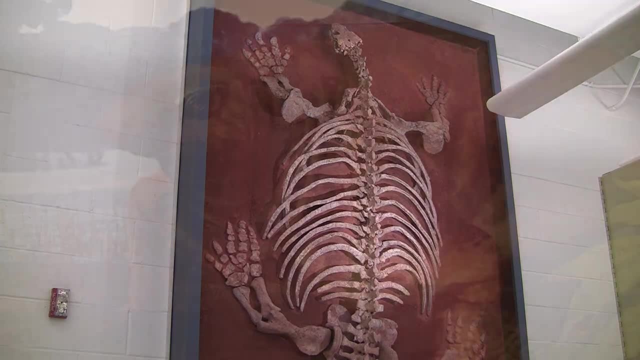 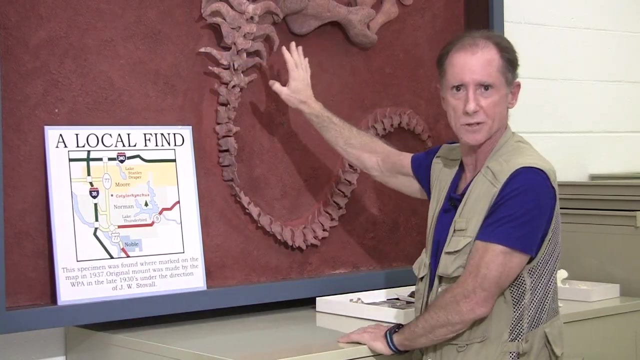 that somebody has never found before. This is one of our coolest fossils. It is something called Cotylerincus. This is from Norman Oklahoma. This is unique to our area. It belongs to a group of animals that ultimately gave rise to mammals- furry things like us. You can see it's got a. 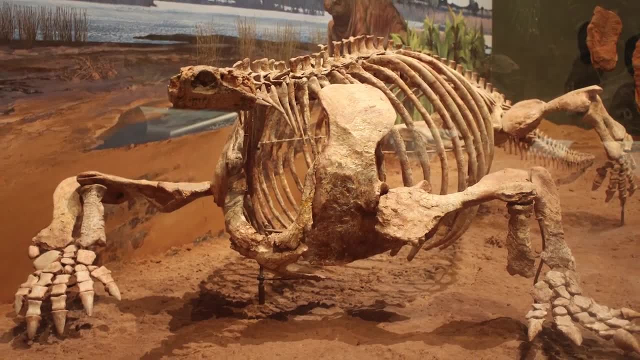 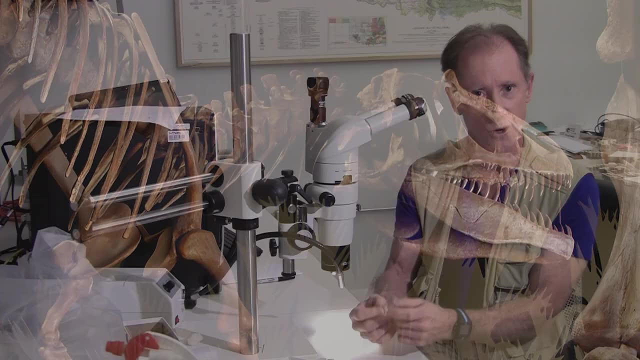 little, teeny tiny head, Great fat body. This was a plant-eating animal. When most people think of fossils, they think of big stuff: Dinosaur bones, these whole skeletons. We also had teeny tiny mammals. On the head of that pin is glued one molar, and that's actually very 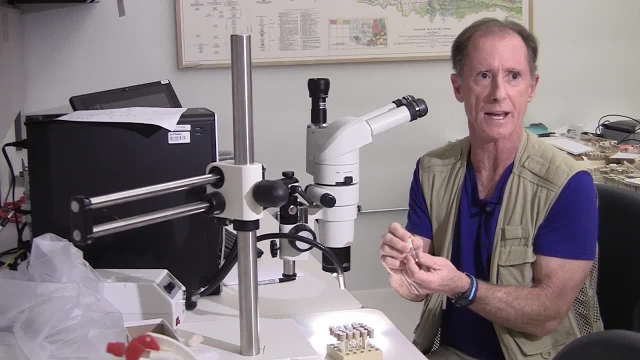 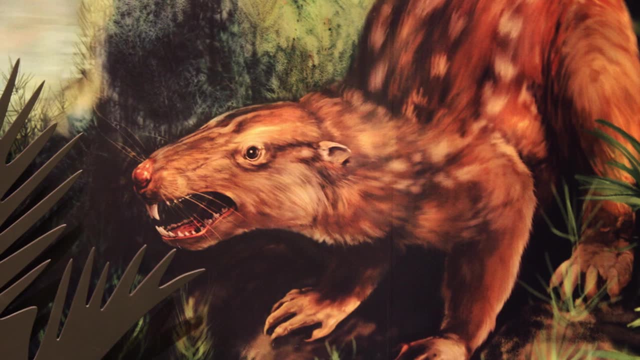 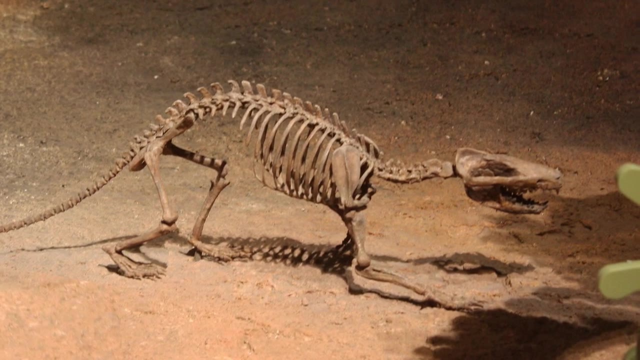 informative. It tells me we had this mouse-sized animal running around southeastern Oklahoma about 105 million years ago, same time as a number of the big dinosaurs, But this was an unusual new species. In fact, all of the mammal fossils we found down there were new. This particular one probably ate insects. 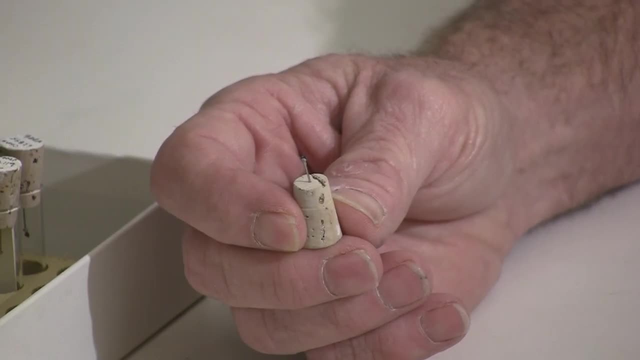 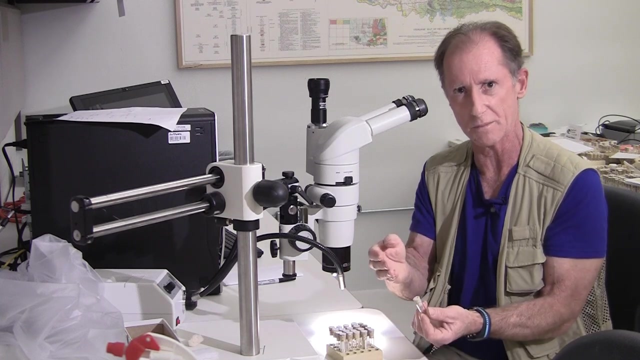 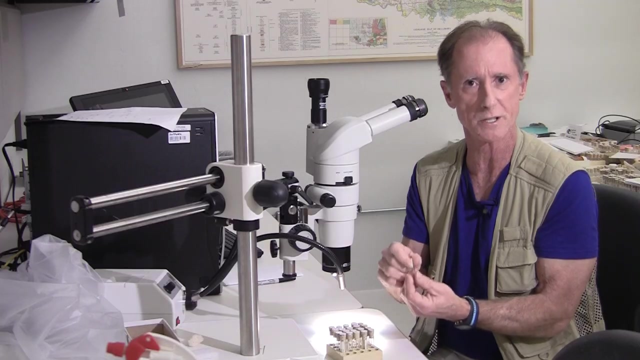 We discovered these things and I had the privilege of naming this as a new species. I named it after our university president. The genus is Atoca thyridium, little mammal from Oklahoma, and the species name Boronii for president David Boron. My name is Nick Ciepleski and I work as a vertebrate paleontologist.